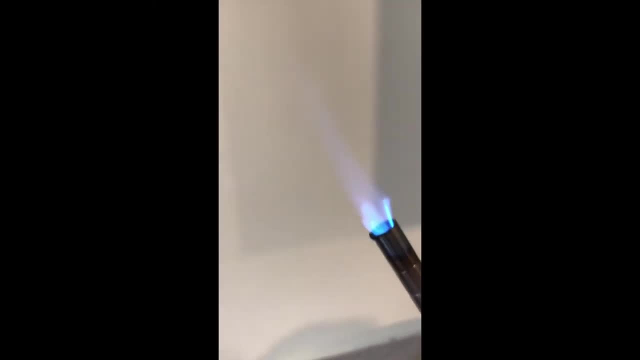 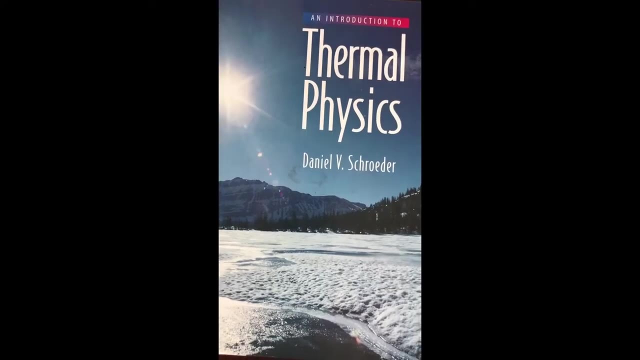 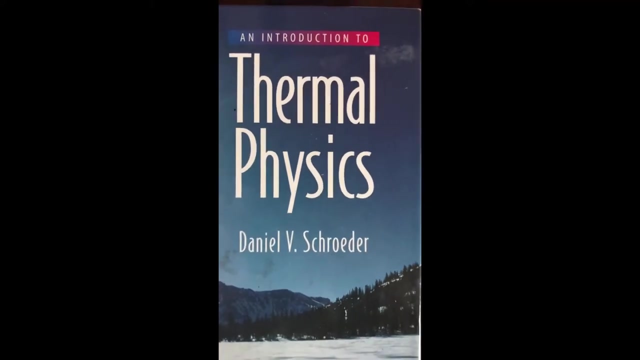 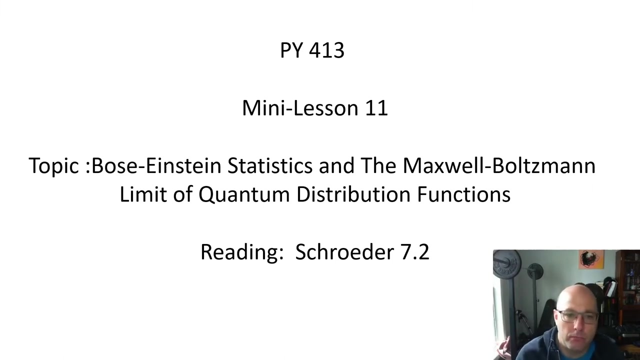 Hi, welcome to mini lesson 11.. In this one we're going to work on doing for a level occupied by bosons the same thing that we did for a level occupied by fermions in the last lesson. So this will be Bose-Einstein statistics, and. 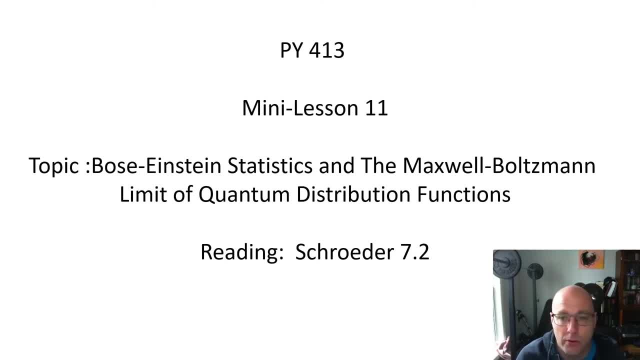 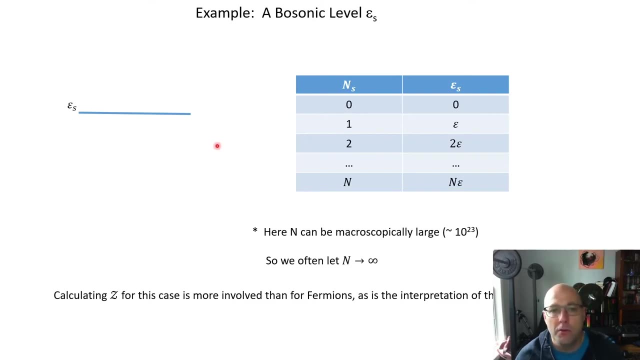 distribution functions, and what we'll see is that this will reduce to Maxwell Boltzmann distribution in a certain limit. So we're still in section 7.2 of Schroeder, and let's look again at our table from a few lessons ago, where we 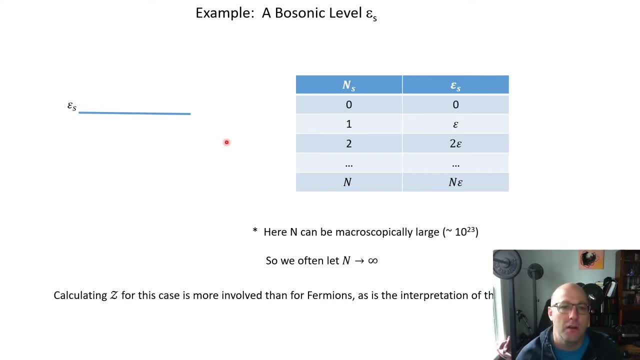 list the possible values of n sub s and e sub s, this time associated to a level that will be occupied by bosons, and so the challenge here is that we have a lot of n sub s, values from 0 up to n, and each one has an associated energy value. 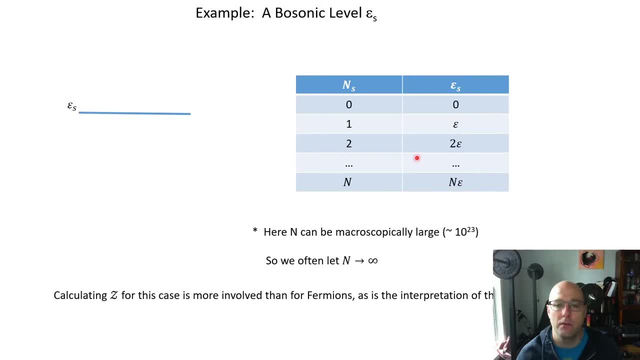 where the energies are just additive. so if you have two particles in the level, it's 2 epsilon. if you have n, it's n epsilon, and so here n can be quite a large number, and so often we let it approach infinity. so because there's so many values in this table, the 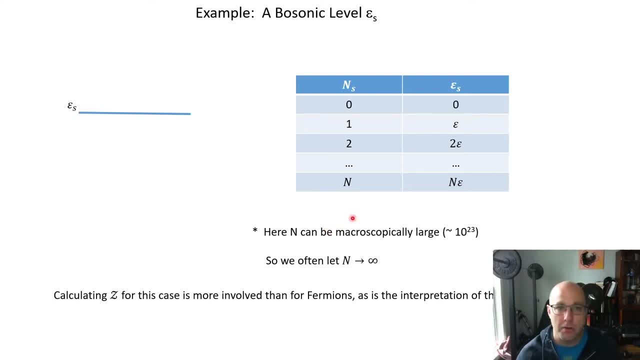 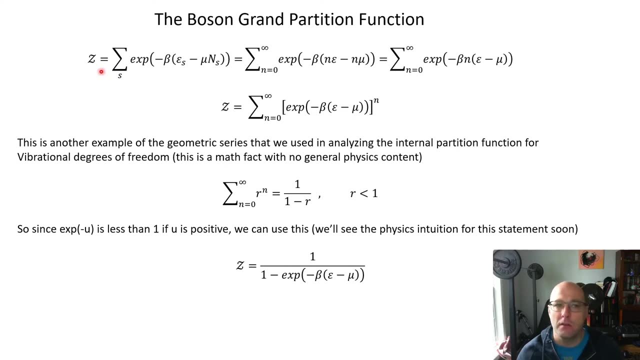 calculation for the bosonic grand partition function will be a little bit harder than it was for fermions, but we can do it. so here we go. this is the definition of the grand partition function, and so letting the number of particles potentially approach infinity. the sum extends from little. n equals 0. 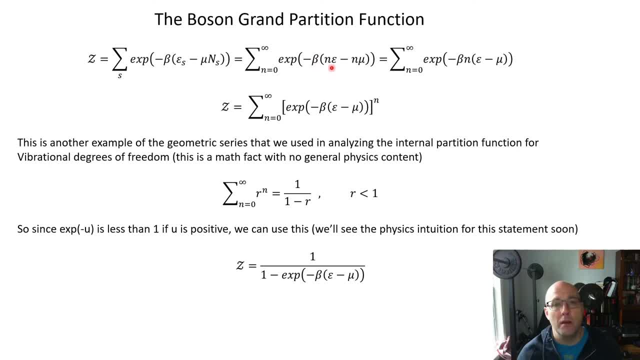 up to infinity into the minus beta. ne is the energy associated to the integer occupation n, and then we get an n month's end. well, little, n is the particle number in this case, and so this sum, we can factor the n out, and that bokeh & write. 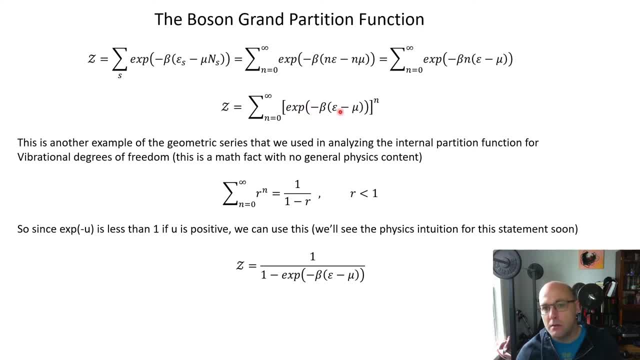 equation you text elephant f, this exponential e to the minus beta S, mod n, give an empty layer, and then you will have two: sacrifice: Jacob X, aj empezek, is equal to the sum from any equal zero to infinity of this exponential, either the minus beta s, and, and then we get an n? mu example, because and little n is the particle number in this case, and so this, some we can factor the end out, and that then reduces also to beautiful: z is equal to the sum from axter by b ist equal to the sum from any equal to infinity of this exponential, either the minus beta s is equal to the value of zo. 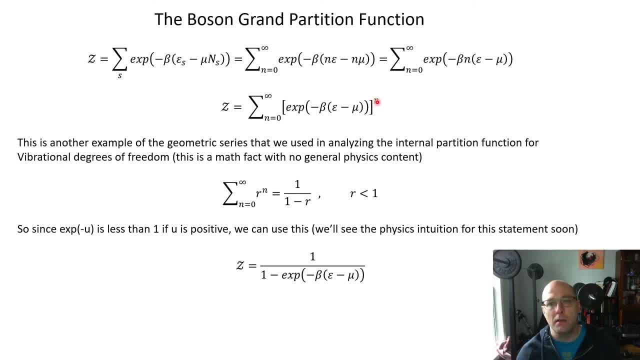 unden hurstd傷ki, epsilon minus mu, all raised to the nth power, right. so just that n in an exponential just pulls out like that. so you might recognize that this is another example of the infinite geometric series that we used when we were talking about the internal partition function for vibrations. last, 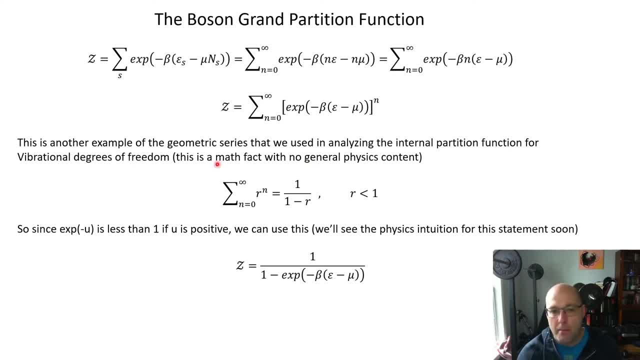 week again. so this is just a math, mathematical fact. there's no physics in here. but sum from n equals zero to infinity of any number. r to the n is one over one minus r, on the condition that r is less than one, and so e to the minus mu is less than one. if mu is positive, we'll see that it is. 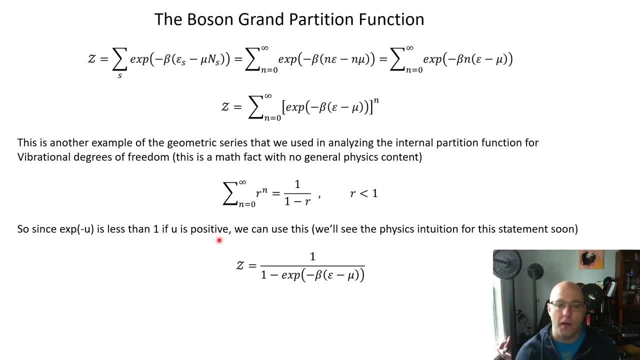 positive in a few slides, and so we can just evaluate the partition function in that sum directly. so this exponential expression is our r value, and so we just get one over one minus the r value for z. so it's not super hard, but it does require you to sort of be comfortable. 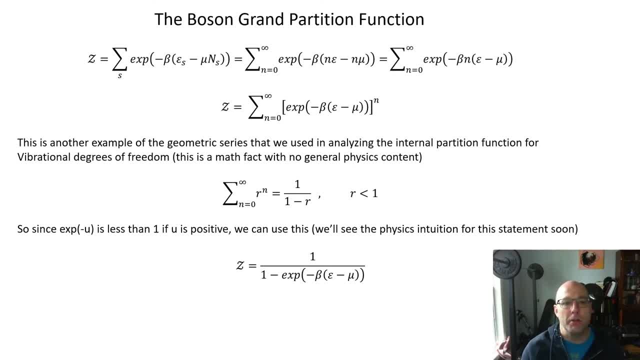 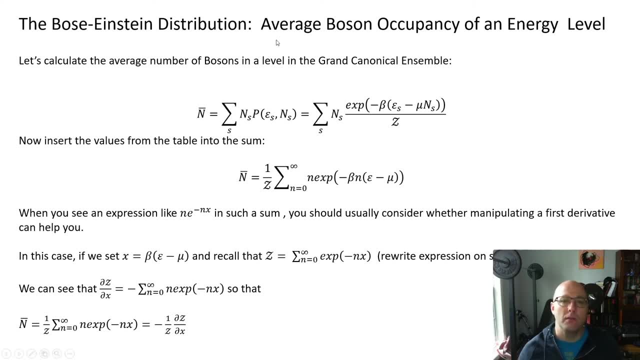 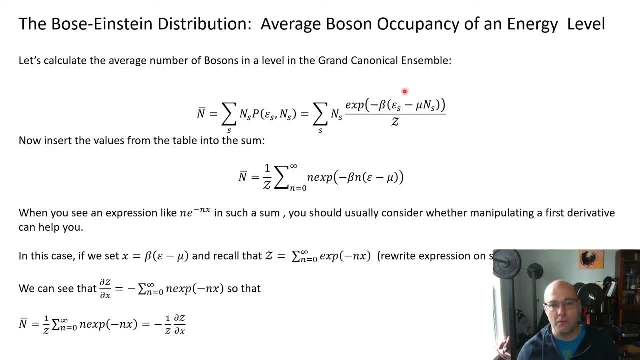 n sub s, and so that's just this expression, which is the gibbs factor, divided, divided by beautiful z, and so we're still going to do that thing where we insert the, the possible values from the table. so now we're going to sum from n equals 0 to infinity, where n is now representing the number. 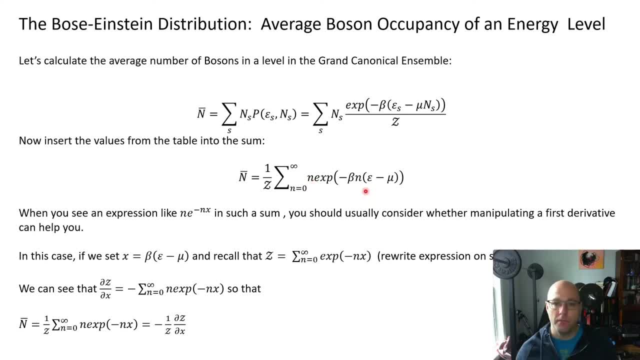 of particles in the system. we have this expression as well, and so, if we look at this expression, this is one of the mathematical slash, theoretical tools that you're really supposed to learn from taking a thermal physics course. when you see, this is my assertion after you've had this course, when 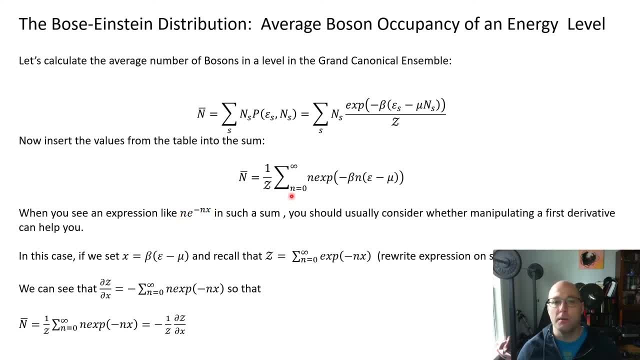 you see an expression like n e to the minus n x in such a sum, you should really be thinking about connecting that to a first derivative as a possible tool for manipulating the sum to your advantage, right? so there's no general rule, there's no thing that says you always must do this, and there's some. 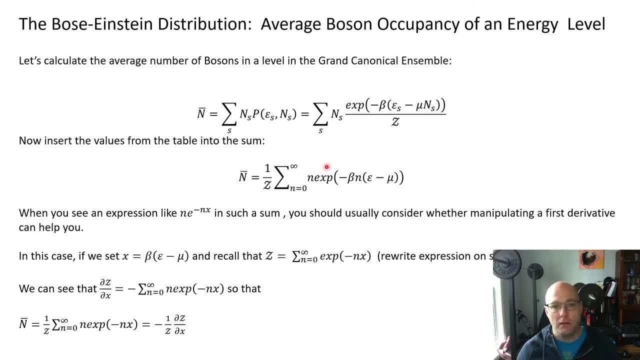 sequence of steps you always have to do, but the basic idea is you should be looking for this. you should be aware that this kind of expression can be dealt with in a certain way and that sometimes it helps you, and that's just one of the tools in your toolbox going forward that you'll be. 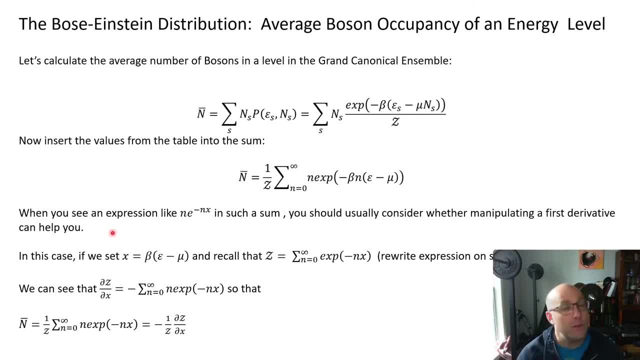 able to apply, even if it's not thermal physics right. so what we can do is set x equal to base theta epsilon minus mu, and so in that notation we'll recall that beautiful z is the sum of n equals zero to infinity, of e to the minus n, x. and so you'll just note that the first derivative of 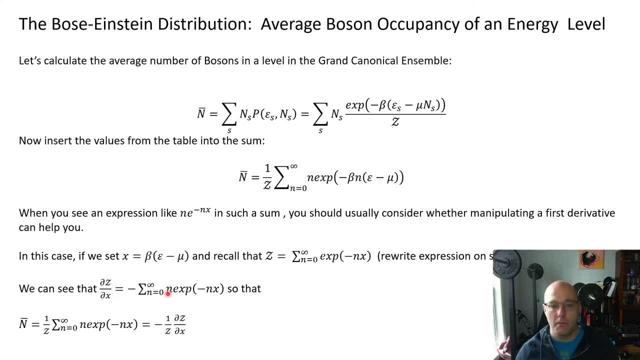 z with respect to x is equal to minus the sum and e to the minus n? x, right? and so what that allows you to do is to write n bar as one over z times the negative of that expression, and that means that n? bar is negative, one over z, dzx, right. so again, what we've done here is to 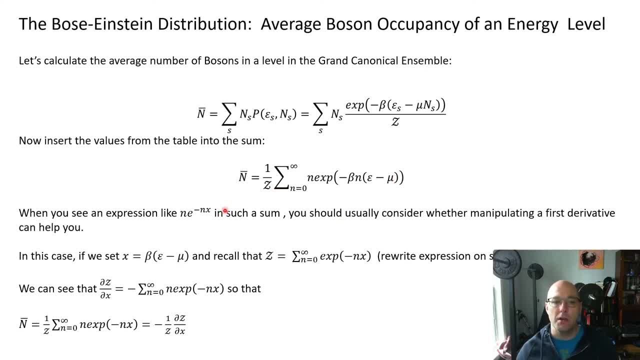 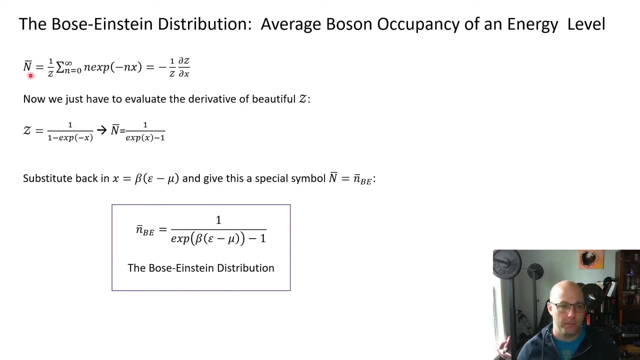 recognize that by connecting this funny expression in the sum to the first derivative of an exponential, we generate a new formula for n bar. that turns out to be easy to evaluate, right? so if we just evaluate this first derivative, where i'm just rewriting the last line on the top line here, so now we have an expression for: 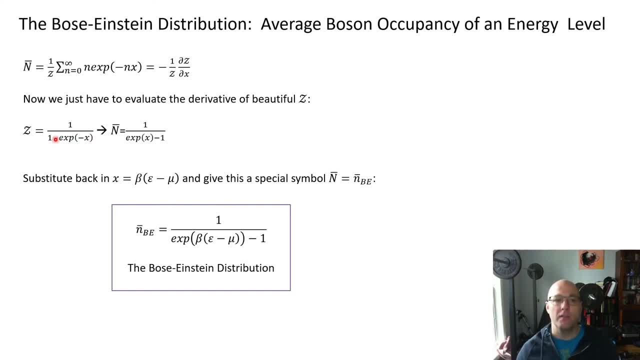 beautiful z from a few slides ago. we can just take the derivative exactly and get this result. so that's just a tool, right? i mean there's not like there's a physics rule that we use. it's kind of it's. i mean, it's a trick, and it's a trick that you should keep in your toolbox. so let's. 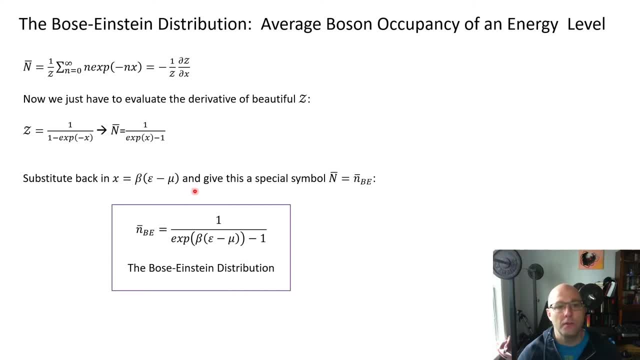 substitute back in x, so that we're back in physical symbols. and as we're going to do that before, we're going to give this average occupancy a special name: little n bar sub b e for bose einstein. so n bar b? e is e to the positive beta epsilon minus mu minus one. this is a bose einstein. 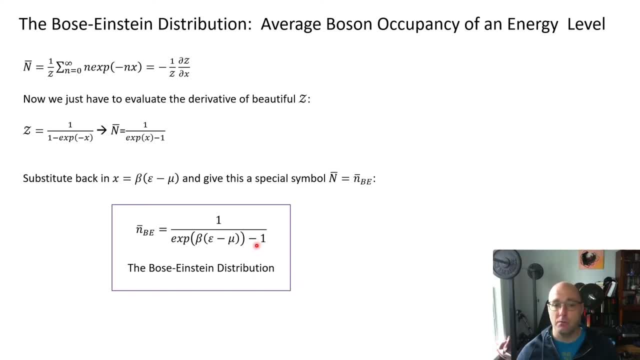 distribution. so this looks just like the fermi dirac distribution, except there's a minus instead of a plus. it makes it easy to remember, but it also makes it easy to mix them up. so don't mix them up. that's a horrible affront to the gods of thermal physics. let's talk about the properties of the bose einstein. 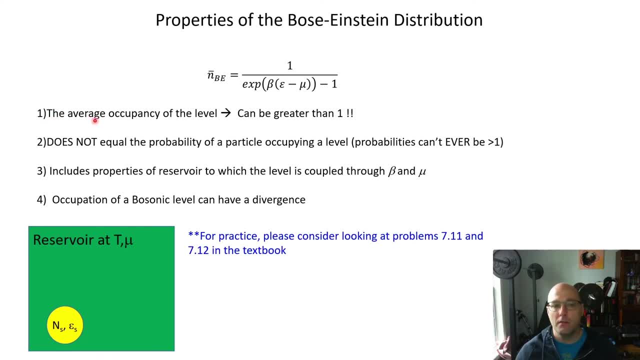 distribution number one: it's still the average occupancy of the level, but in this case it can be greater than one. right, because average occupancy? because the occupancy of the level can be anything from zero up to infinity. this number can be whatever. it can't be negative, that doesn't make any sense. 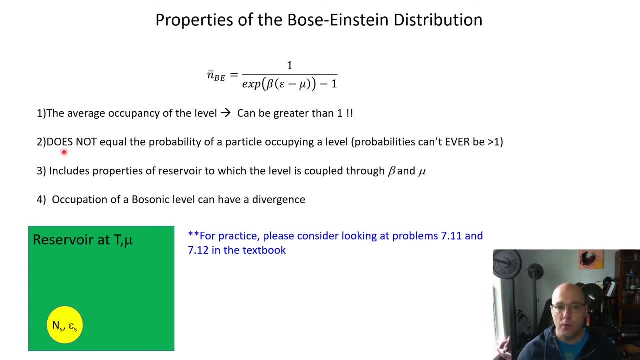 so because it's always because it can be greater than one, it is not in general equal to the probability of the particle occupying a level right, because the probability can never be bigger than one and that's an important distinction. so, if you remember, in the mini lesson about fermi, 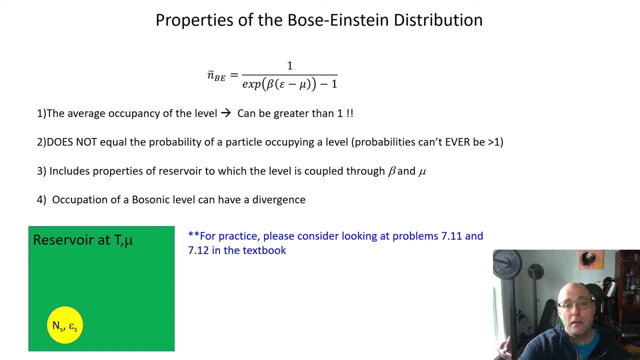 dirac statistics. i made the point that the fact that n bar fermi dirac was also the probability of occupancy was only applicable to fermions, and this is the probability of occupancy of fermions, the case where you can see that it's clearly not a general fact. all right, it also includes the 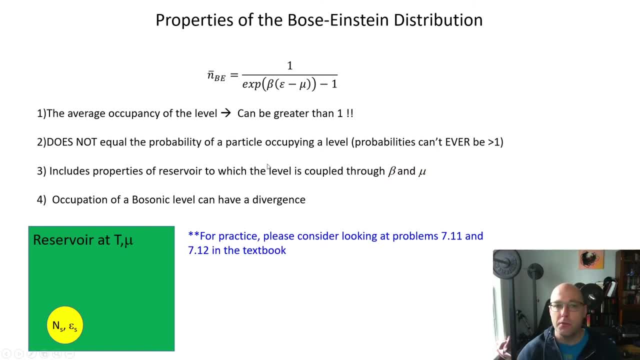 reservoir properties of temperature and chemical potential. the most important property of the bose einstein distribution is that it can clearly have a divergence. if e to the beta epsilon minus mu equals one n bar b e diverges, that's really significant. it means basically it means there has to be a phase transition. so we'll be talking about that later. 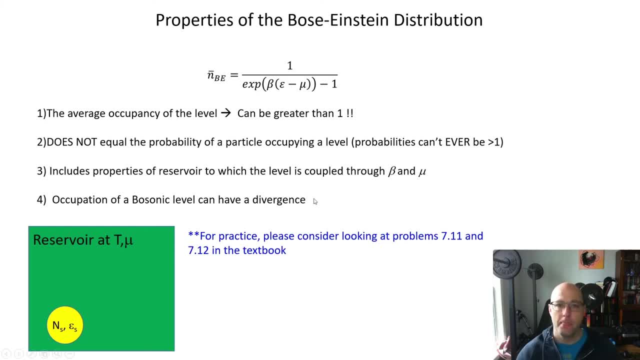 in the context of the bose einstein condensation. but it also shows you why we're able to accurately get away with using the geometric sum, because this e to the minus beta, epsilon minus mu, was our ratio in the geometric sum, and the case where epsilon is less than or equal to mu means you've. 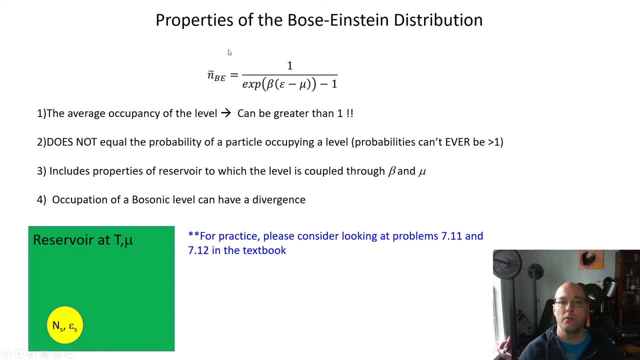 crossed over a divergence and that's completely non-physical. so we're we. we can sort of a priori understand why we were sorry, a posteriori understand why we were able to use the geometric series without getting into trouble, that the ratio might, that might, be bigger than one. so for practice, using the fermi, dirac and the bose, 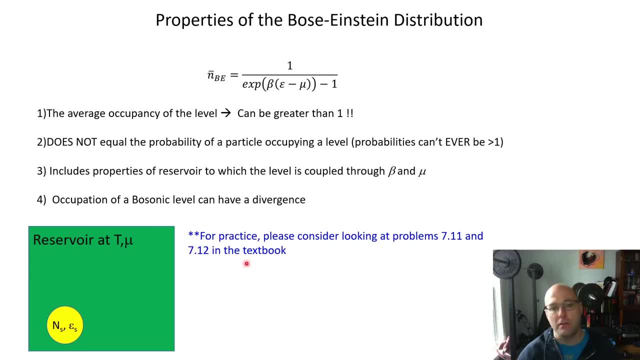 einstein distribution. i think you should look at problems 711 and 712 in the textbooks. they're really plug and chug examples there. there's nothing particular about them, but they're really tricky about them, um, but it is useful to go through them so that you're just comfortable. 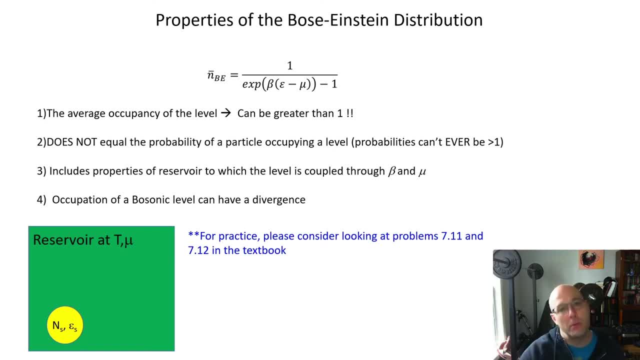 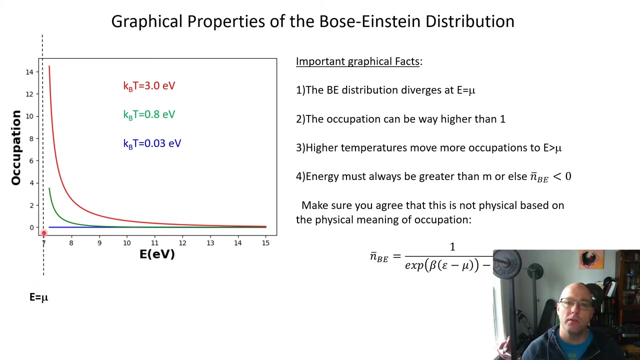 using and thinking about occupancies versus probabilities, etc. etc. um, and i will have solutions to those posted, even though they're not technically assigned for the week, as homework. all right, so let's keep going with graphical discussion. so again, when epsilon equals mu, the bose einstein distribution has a divergence right and it actually decays pretty rapidly. 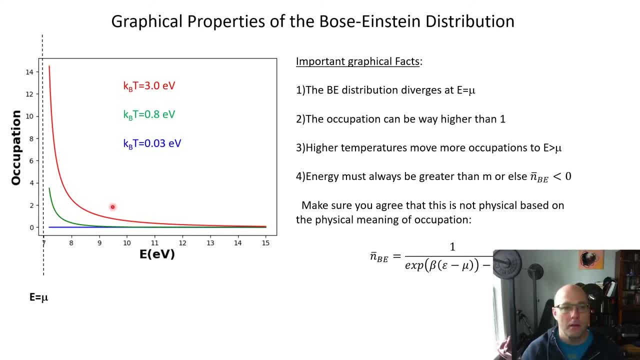 away from there. um, as you can see, the occupation can be way, way bigger than one. you know, as you approach mu, it approaches infinity. as you go to higher temperatures, you have higher occupancy at energies above the chemical potential mu, right. so it gets so low- there's almost so- at low temperature in the blue curve there's almost no occupancy at adv. 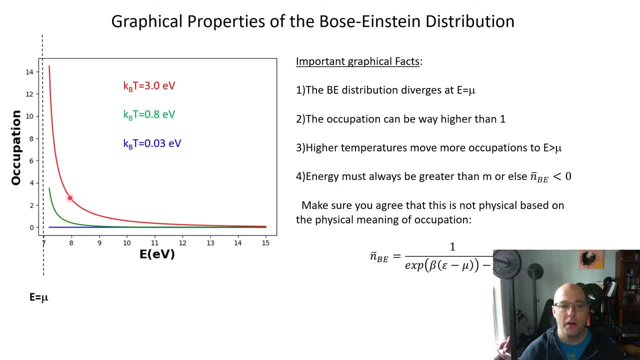 and then as you increase temperature, the occupancy at that high energy goes up and up, and up and up. all right. and so one thing that we know is that the chemical potential is a is a lower bound on the energy, so energy is always greater than that energy below the chemical potential. that should be immune, not an m. 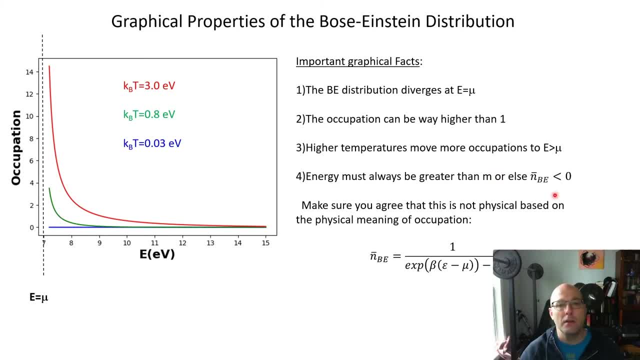 it's not physical, but as you go, style $$$. estoupeou à ça au mental qui continue à plusاه. physical, because it would lead to a negative occupancy and a negative average occupancy makes no physical sense. you can't have a negative number of particles in a level all right. 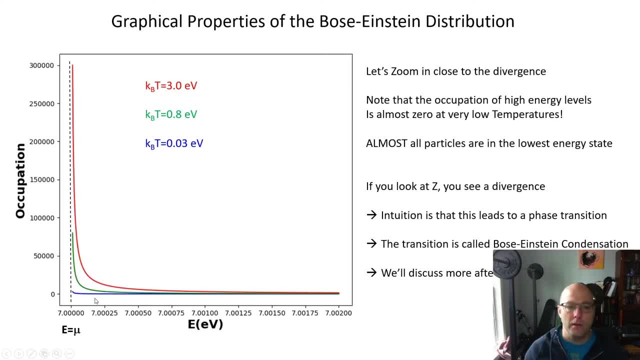 so let's just make one more point. we're zooming in really, really close to the divergence for these same same temperatures. so, look, the y-axis scale has gotten huge. um, the thing i want to say here just by looking at this, is what fraction of particles are in the lowest energy state? 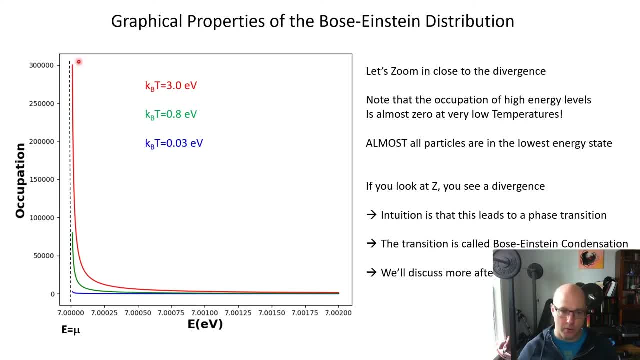 right up on the chemical potential is a really important question, and so the basic idea is: look at the blue curve. in the blue curve there are there's almost no occupancy, even kind of close to the divergence. over here. you just see a slight upturn, right, what that's telling you is really all of the particles at low temperature. 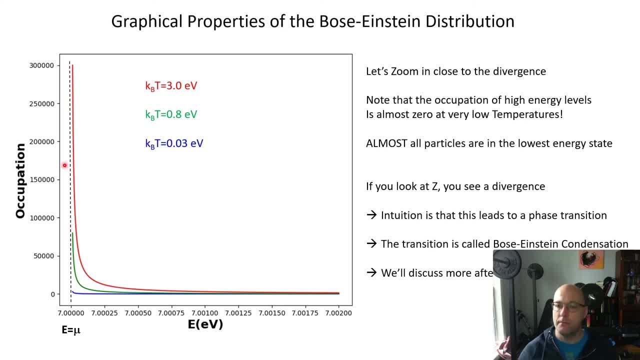 are just falling into this lowest energy level, right um, and this is a characteristic of this phase transition, but basically, as you lower and lower the temperature, a larger and larger fraction of all the possible particles are in this one energy level and basically behave as one quantum wave function possibly containing, you know, 10 to. 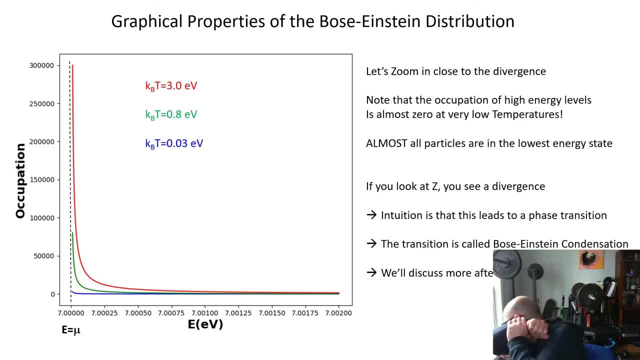 the 23rd particles. jeez, sorry. all right, so we're going to do both einstein condensation in some detail after test two, um, but hopefully the this idea that that all the particles are occupying this lowest energy level is already apparent graphically. so, once again, i almost always give. 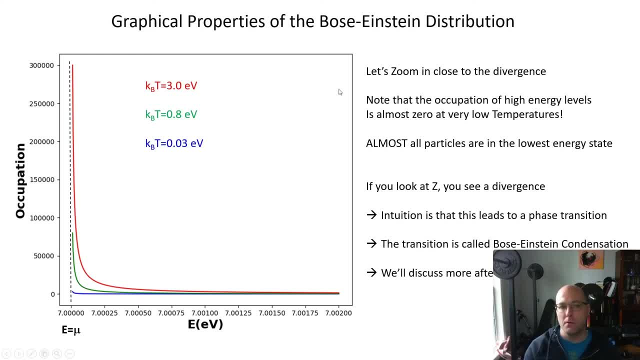 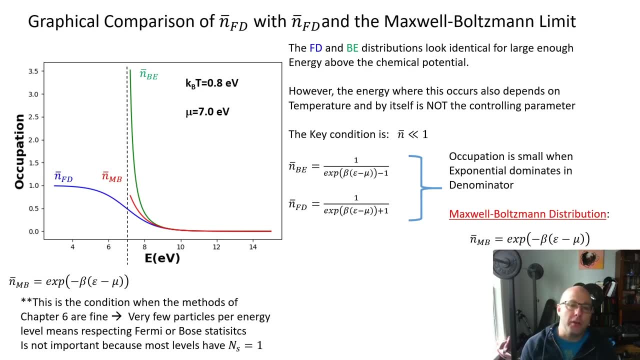 graphical questions about this quantum statistical distribution functions, because i think that's where a lot of your physics intuition comes from, and so here's an example of that. i'm going to plot fermi-dirac and bose-einstein. fermi-dirac is in blue. that's the little step function. 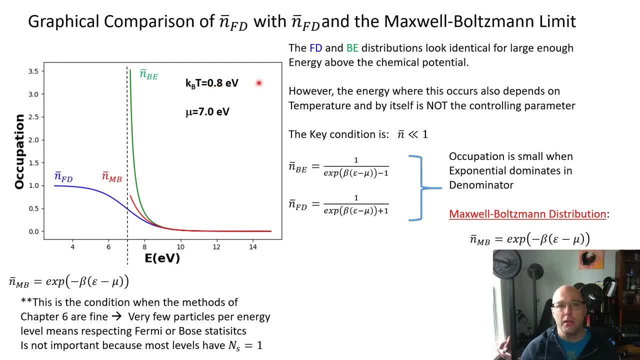 i plot it for a pretty high temperature, so kbt is 0.80 v, which is super hot if you calculate the temperature in comparison with room temperature. right? um, for bose-einstein i use the feeling that the temperature is not going to be very high. so what i've done is i've made a 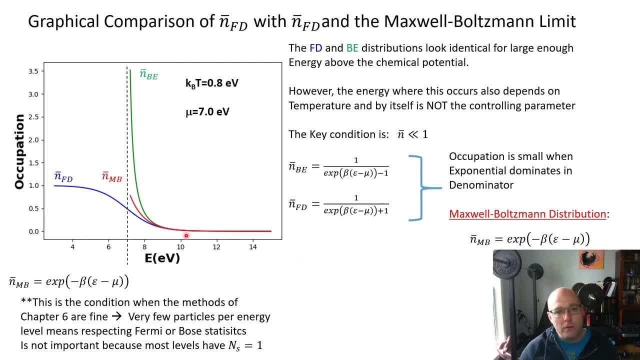 little pure here. this- and i've used that to make my or. the other thing here is that for a certain temperature i can go whatever temperature i want. terms of energy. it's not necessarily energy that's the key here, but it's rather the y-axis. 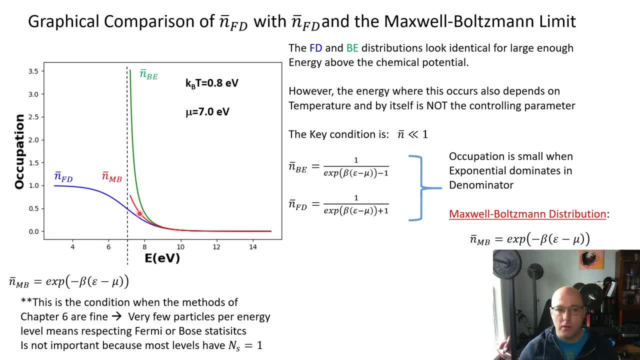 that's the key is that as the occupation goes substantially less than one, these curves are overlapping. The question of what energy matters sort of depends a lot on chemical potential and really the controlling factor is the occupancy. So if we consider the idea that 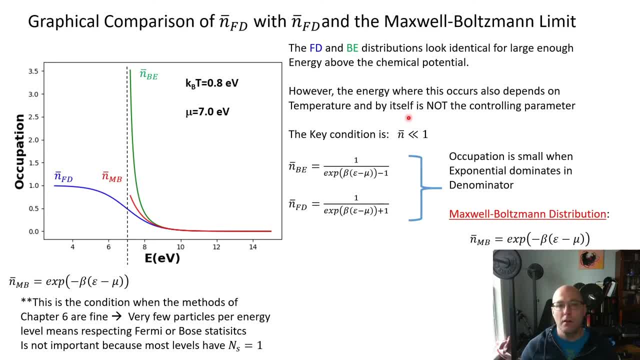 Fermi-Dirac and Bose-Einstein distributions agree with one another. they're the same function for occupations much less than one. you see what happens To get an n-bar much, much less than one. you need the exponential in the denominator to sort of be. 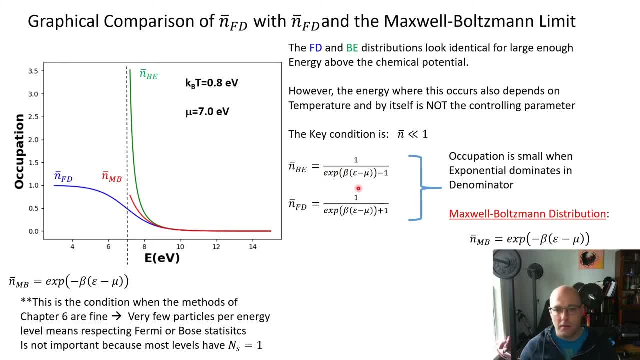 the dominant term. So, in other words, this exponential needs to be much, much greater than one, so that the denominator is huge and therefore n-bar is small, and so that means that whether you have plus one or a minus one in the denominator,